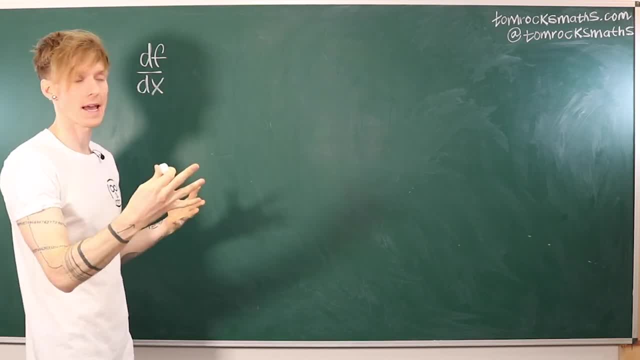 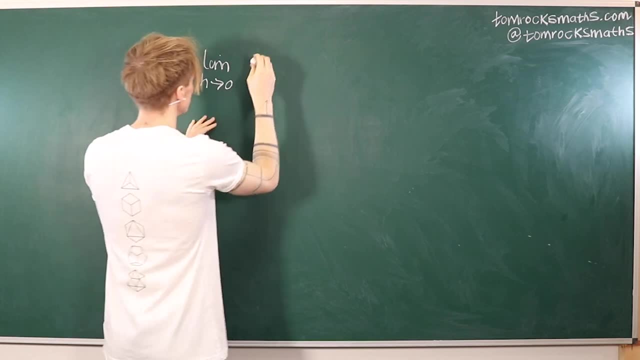 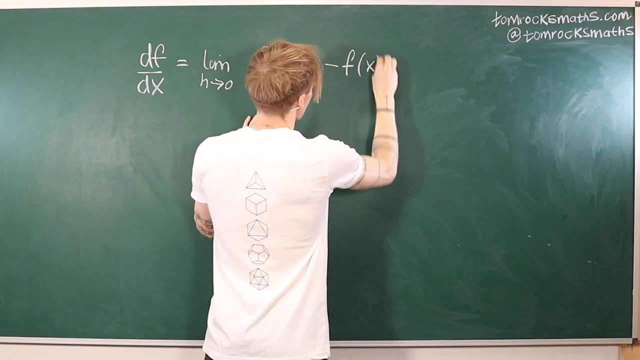 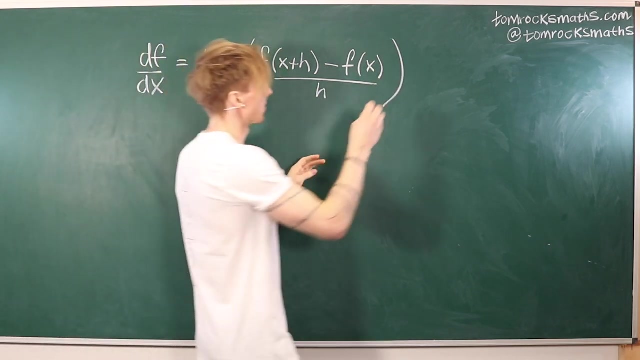 for a function, f of x, then this is equal to the limit, as h tends to zero, of f at x plus h minus f at x divided by h. If we were to look at the graph of this function, which maybe would be something like the following: so f of x. 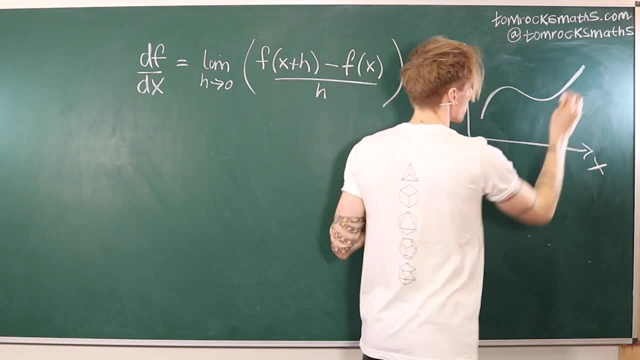 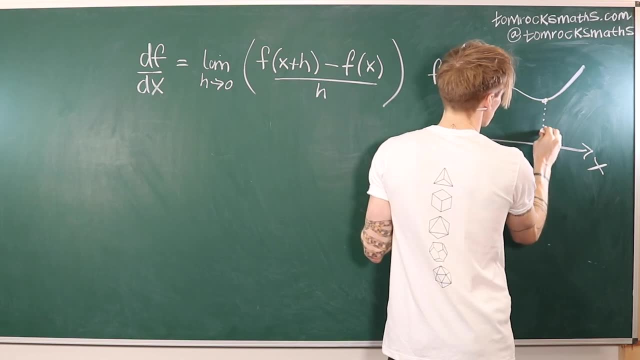 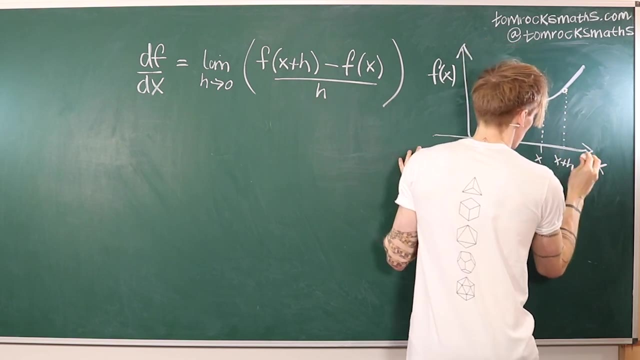 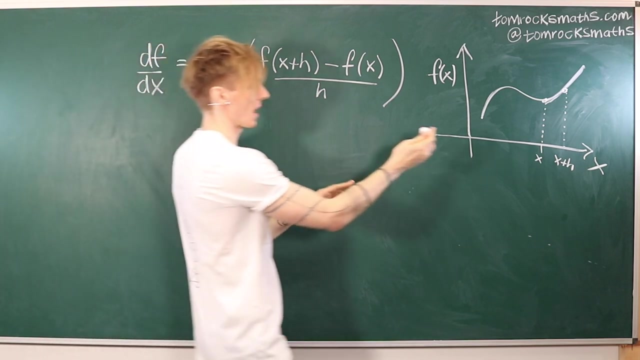 and then x. perhaps it would look something like this then. what we're doing here is we are taking a point here- let's call this x, another point at x plus h, and what we're doing is we're approximating this gradient and we're taking the limit as we allow this point to move closer and closer to x. 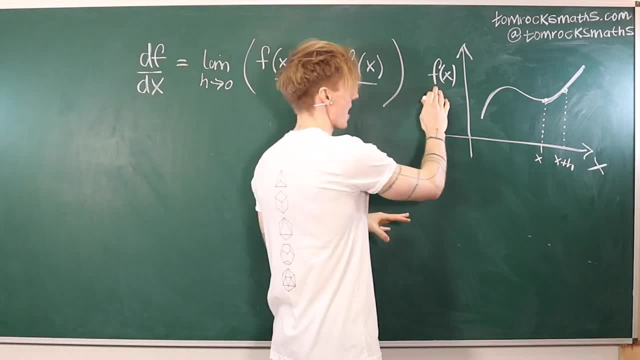 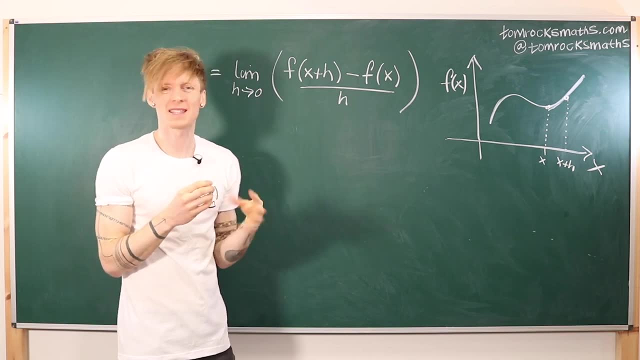 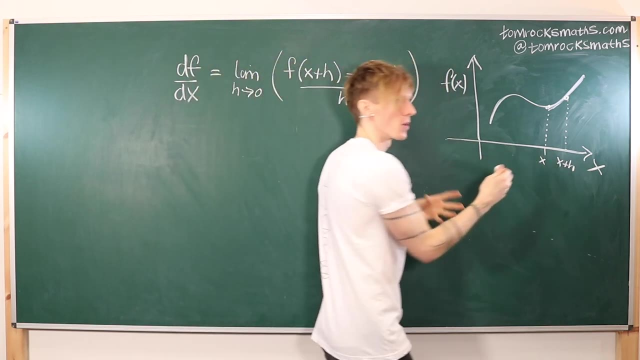 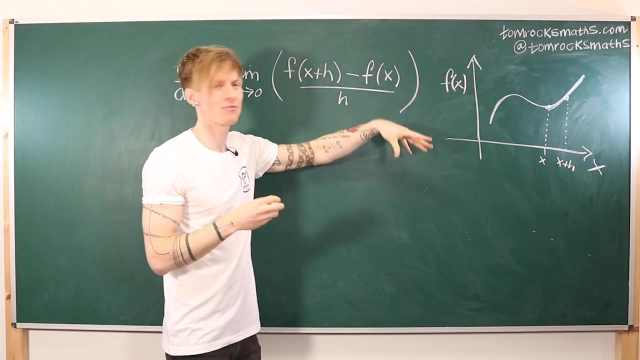 So we're working out how does our function f change in the x direction, Because f is just a line. what this means is that f can only change in the x direction. So as we move along the x-axis we're interested in how does the value of f or the value on the y-axis change? So the only 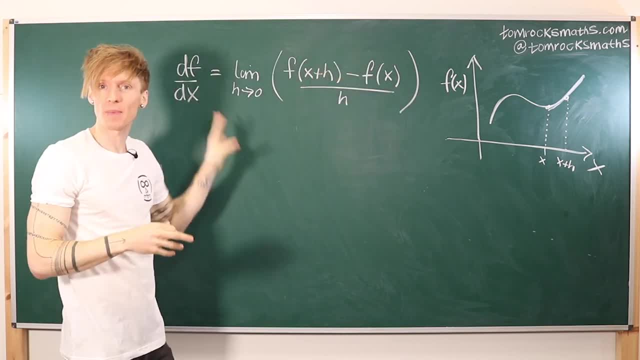 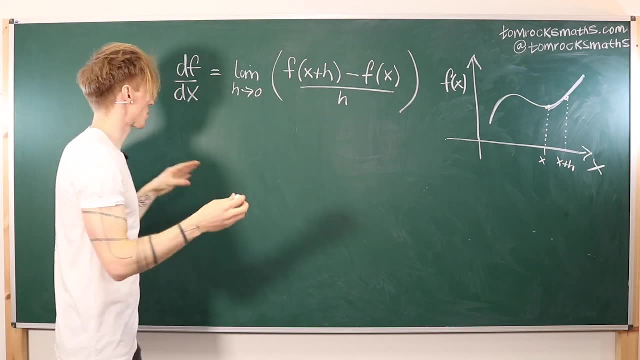 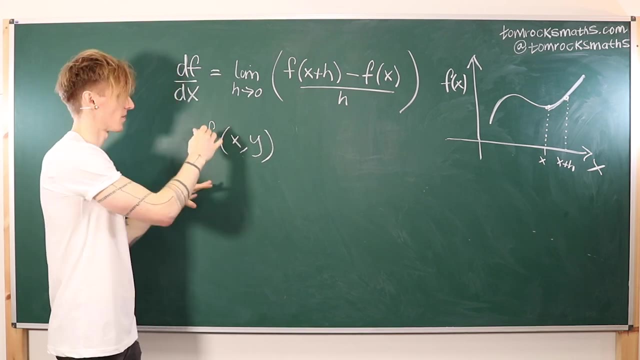 real derivative we can do here is df by dx, because that is the only direction in which f is changing. Now, if we have a function of several variables- and let's just start with 2, for example, we have f of x and y, So now f depends on. 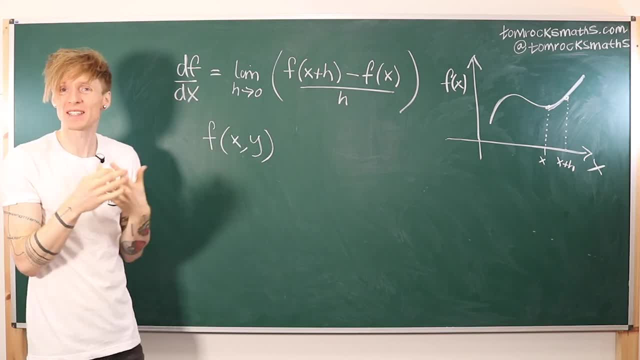 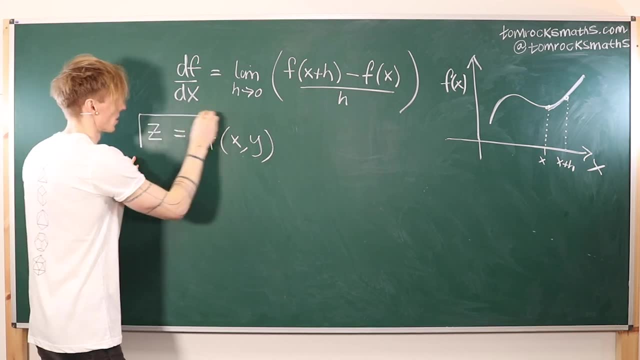 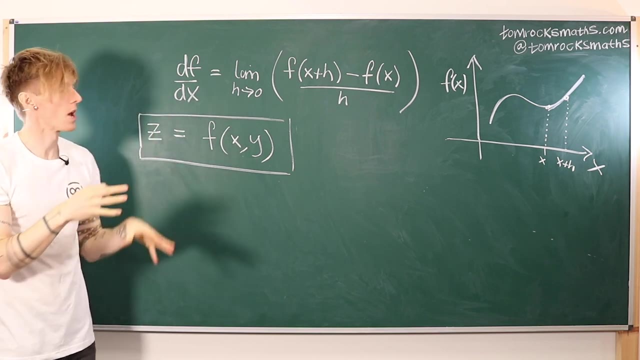 both x and y, and so what this is actually going to give you is a surface. So if you were to plot, z is equal to some function of x and y. you get a three-dimensional surface which will change in both the x direction and the y. 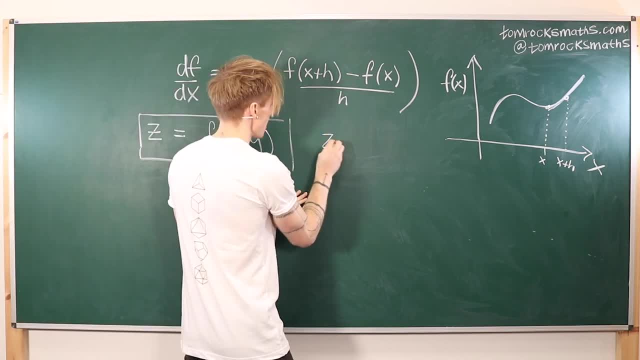 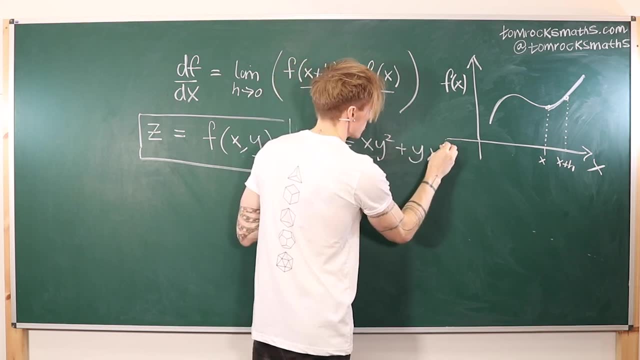 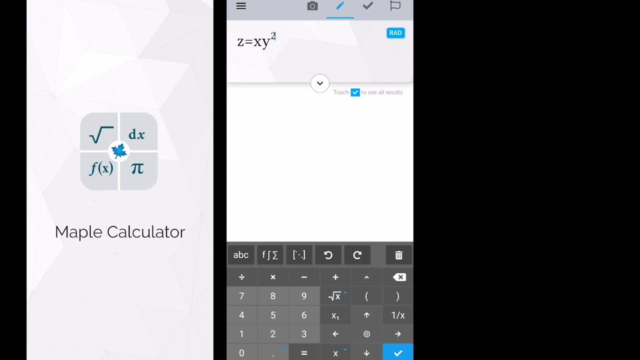 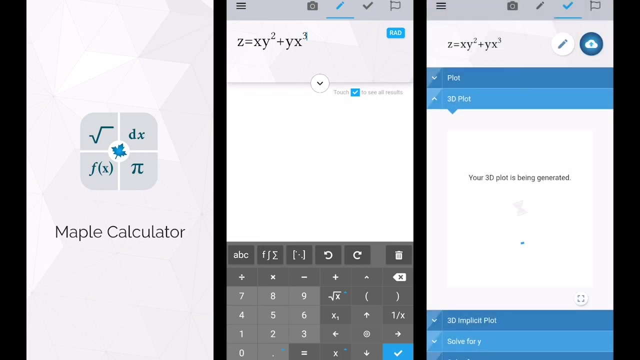 direction. So if we consider the example, z equals xy squared plus yx cubed. So when we plug this into our maple case calculator app, we are given the three-dimensional surface plot of this function and we can see that it is indeed a surface. It's changing in both. 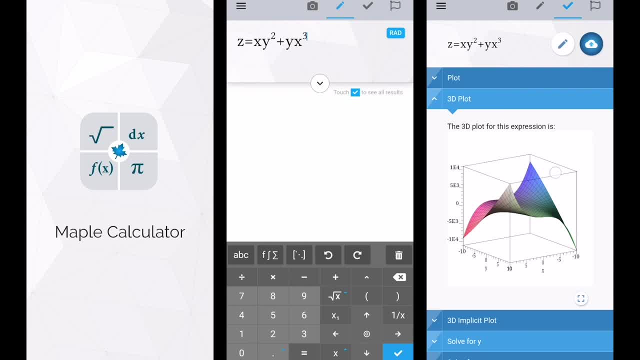 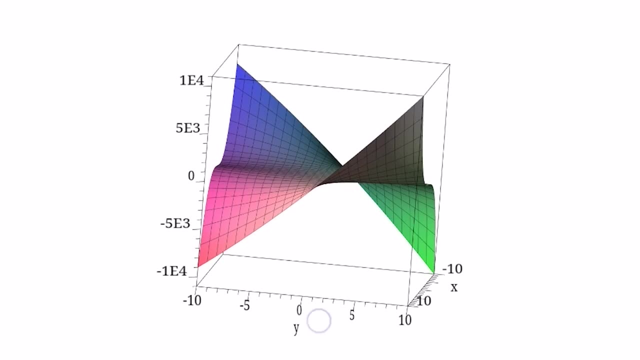 the x and the y directions simultaneously, and so, therefore, it now makes sense that you might want to know how the function is changing in more than one direction. As an example, from this particular viewpoint, we can see that as we move along the x-axis, the function is: 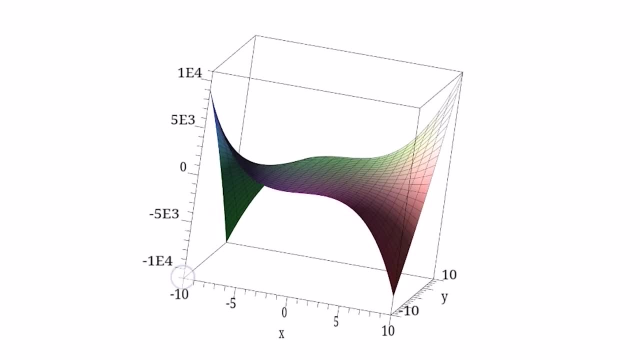 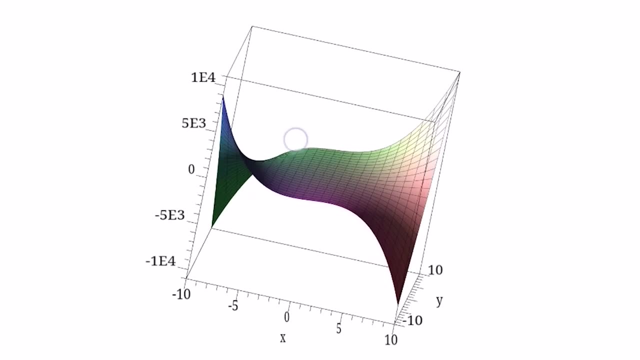 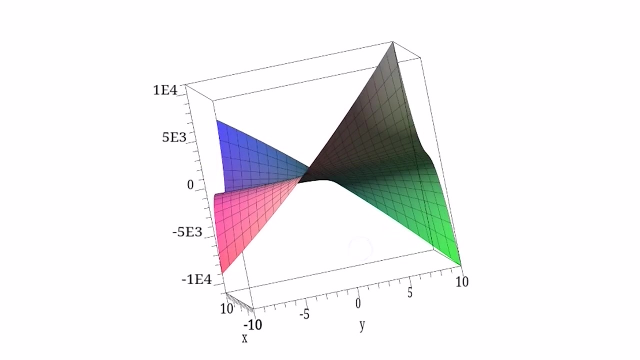 decreasing. so in this direction, in the x-direction, our function is decreasing. But if we rotate the image we can now see that along the y-axis, so in the y direction, our function is increasing. So our function is behaving differently it. 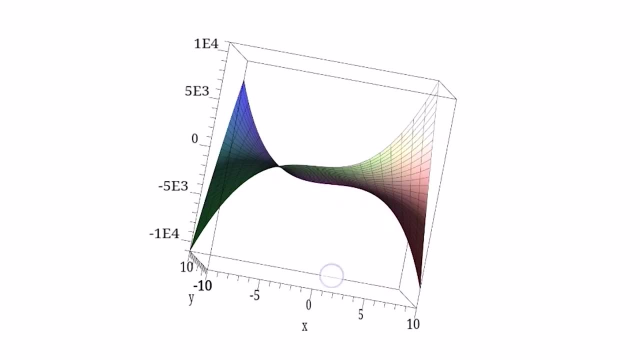 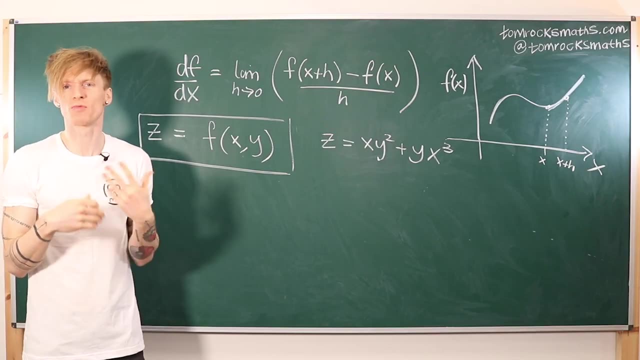 is changing in a different way depending on the shape of the surface and so the direction in which we are investigating. And so what partial derivatives really do is allow us to calculate the rate of change for a given direction. So the x partial derivative tells us how does our function f of x, y 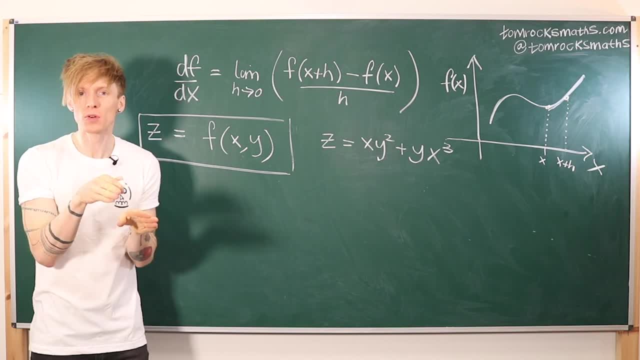 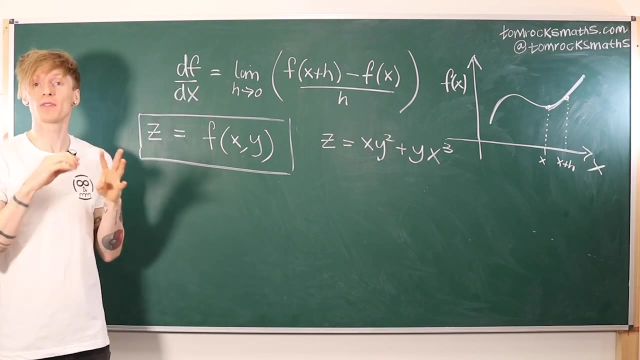 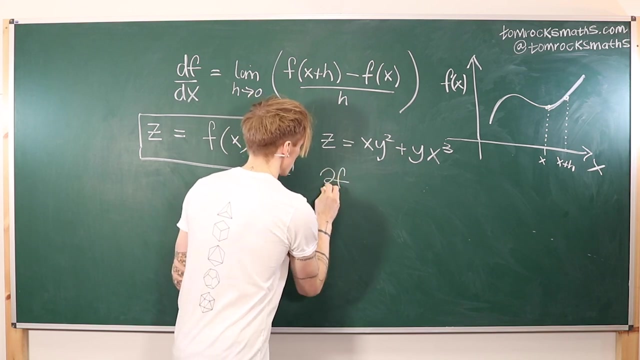 how does that change, specifically moving in the x direction? And then the y partial derivative will tell us how our function changes if we only move in the y direction. So mathematically, our definitions are going to be as follows. If I want to know the partial x derivative of f, where f is a function of: 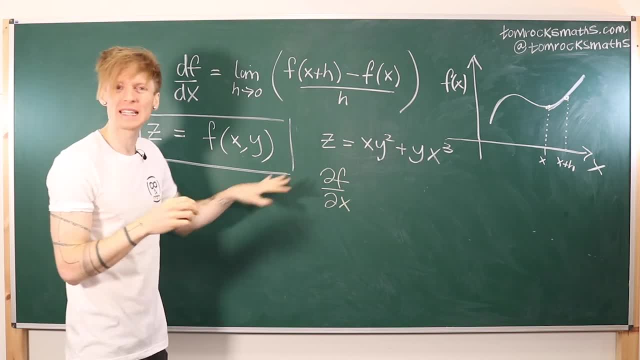 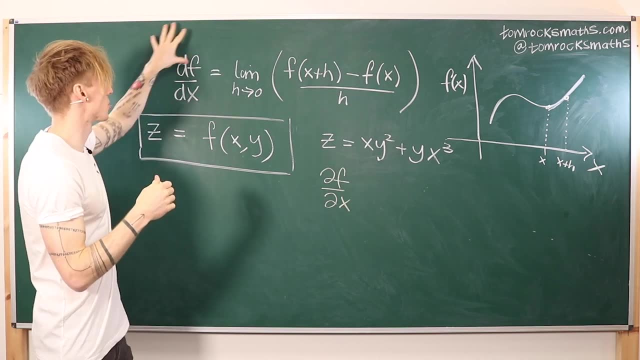 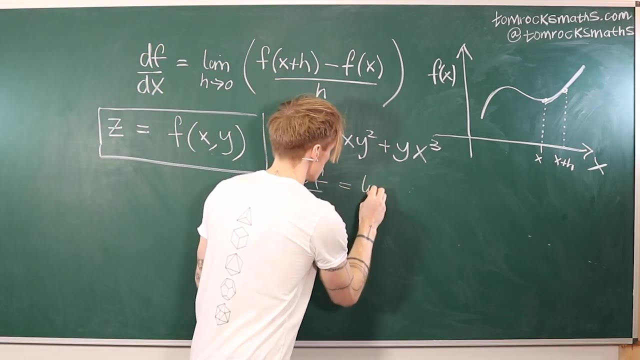 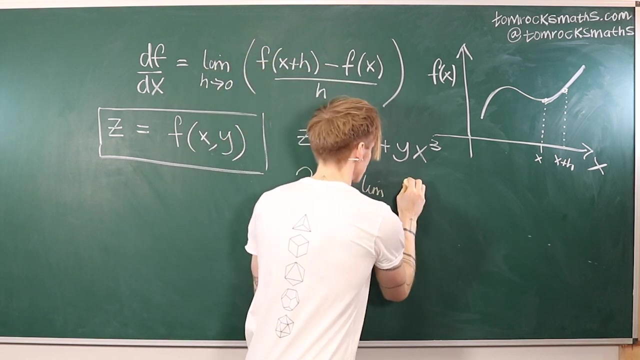 x and y. first of all, we use this curly D notation and this just says that this is a partial derivative Compared to the standard or full derivative in this situation, And we define this to be the limit, as h tends to 0, so unchanged so far, of f of x plus. 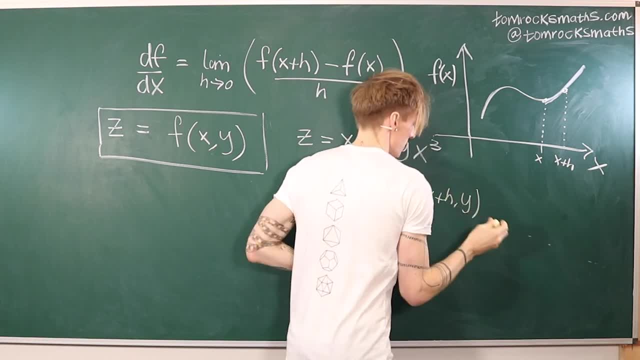 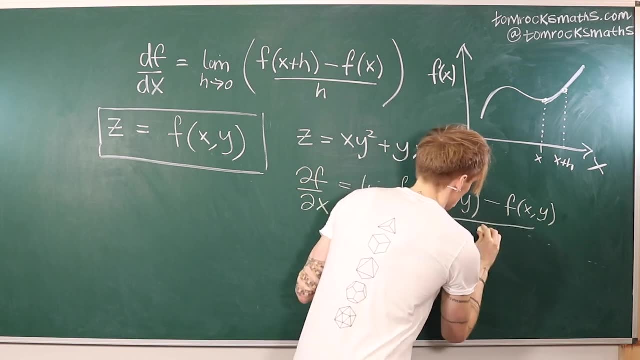 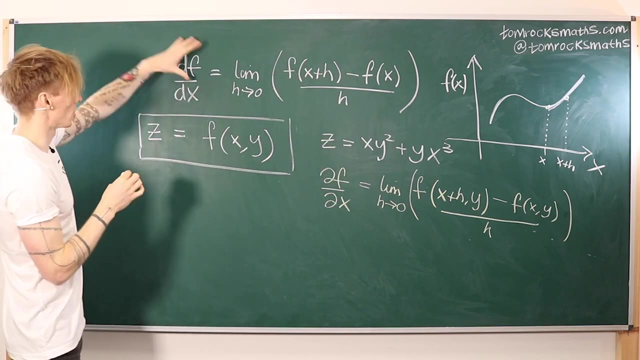 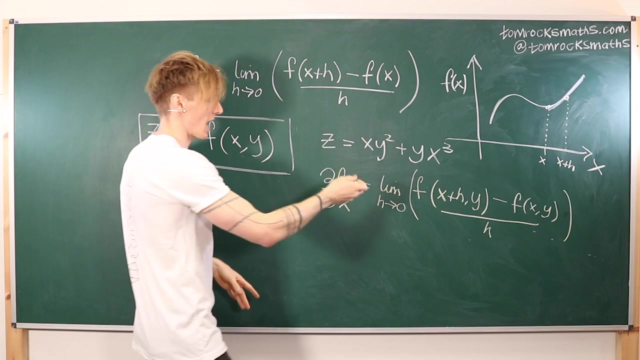 h comma y minus f of x- y, all divided by f of x, plus h comma y minus f of x- y, all divided by h. So you'll notice it's very similar, in fact almost identical, to our full or standard derivative df by dx, But in the partial case what we're doing is we're 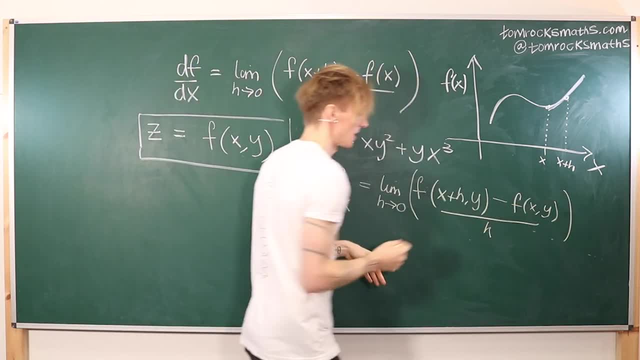 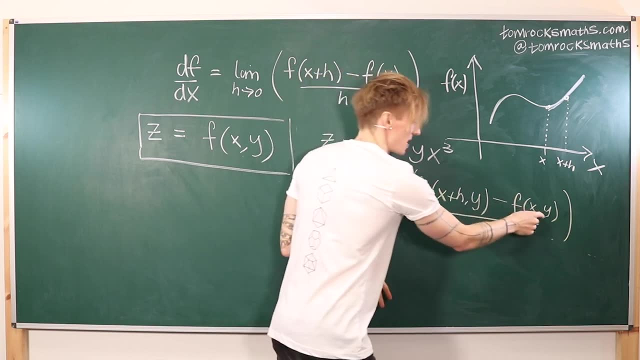 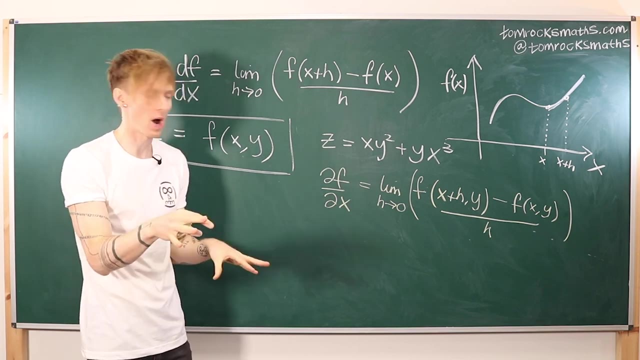 adding our h, our small increment. this is added only to the x coordinate of our function. y remains unchanged. So this is telling us that the y coordinate doesn't change. The value of y remains constant. And we're just looking at what. 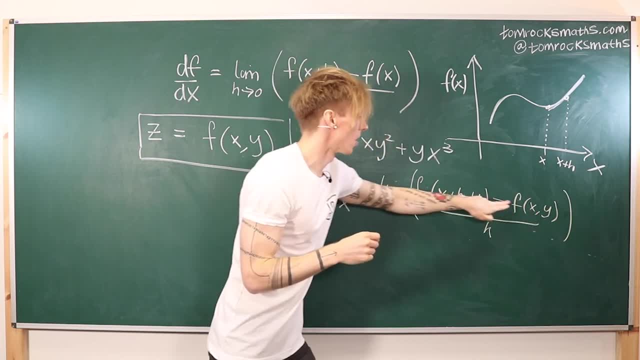 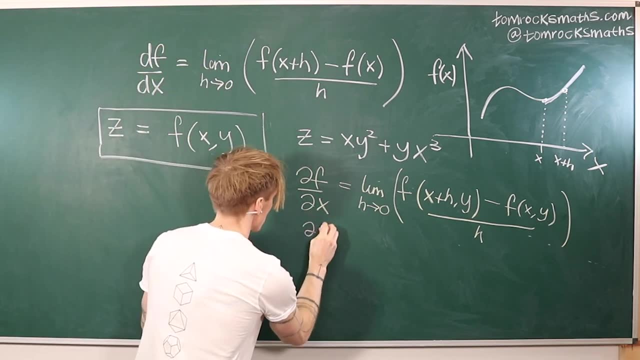 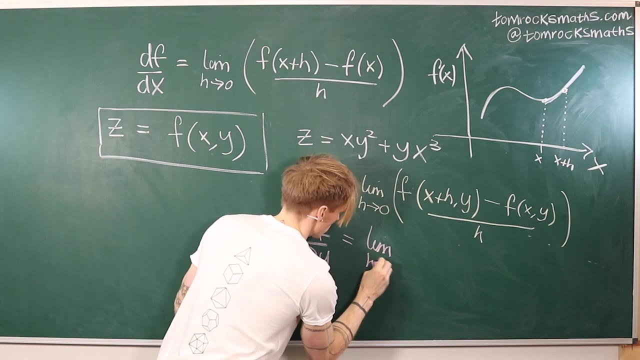 happens if we change the x value only. The partial y derivative is of course very similar. So here we're interested in how f changes in the y direction. So we take the same limit as h goes to 0, but now we leave x unchanged. 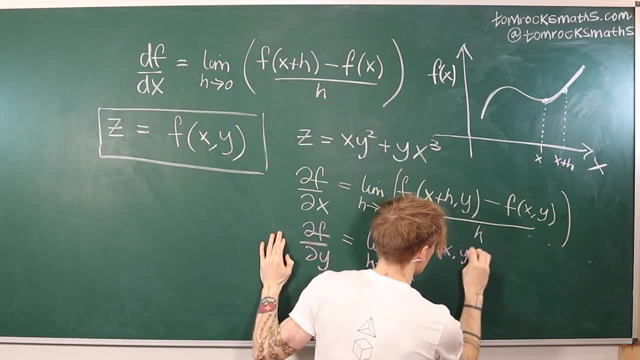 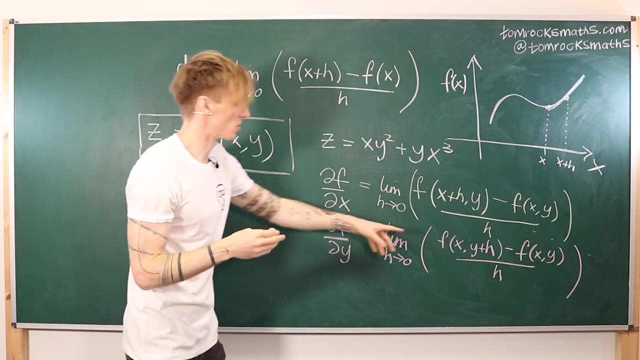 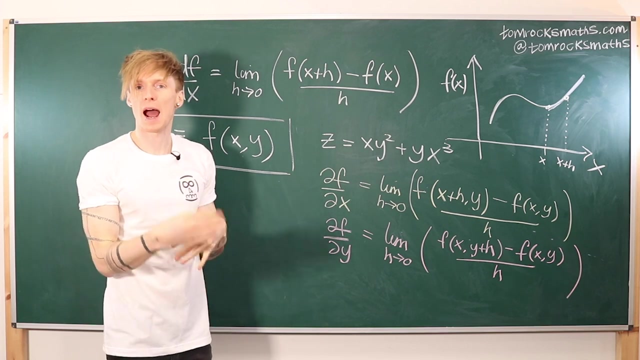 So it's f of x, And now we add h to the y value, then we subtract f of x, y and then we divide by h. So very similar to the partial x, except now we do the plus h on the y coordinate because we're interested in how the function changes. 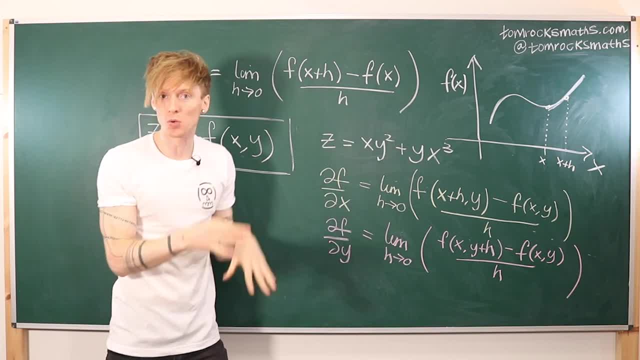 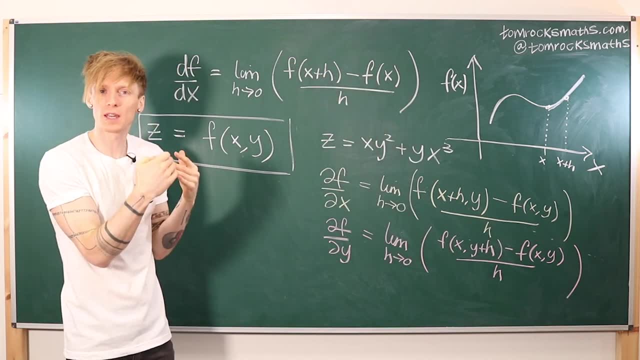 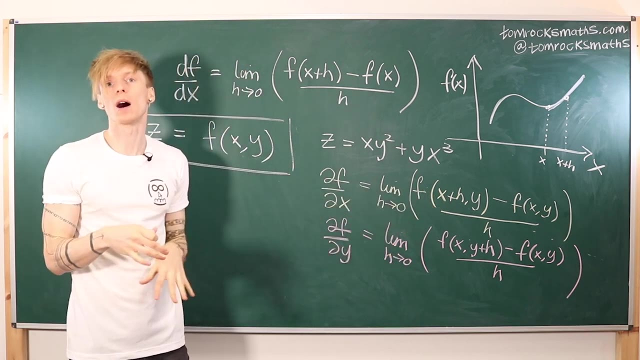 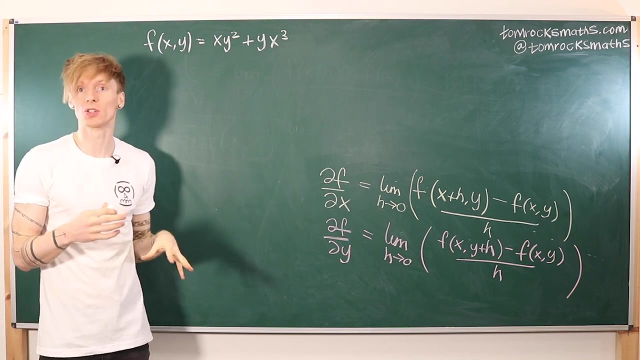 when we change y and only x Finally change y. So the x coordinate here remains constant and we are purely moving a small amount in the y direction and then taking the limit to calculate the y partial derivative. Now that we know the formal mathematical definitions of our partial x and y derivatives, 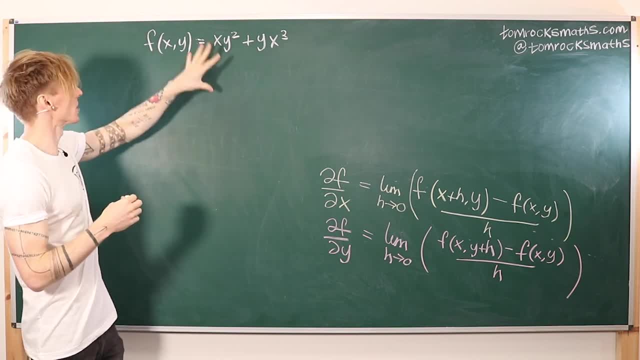 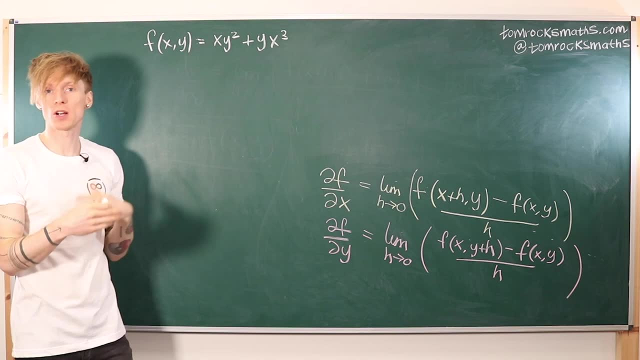 let's actually work through an example of the function we looked at earlier. f of xy is xy squared, So let's compute the partial derivatives to see how this works in practice. And the key thing here is to remember that when you're doing your x partial derivative, 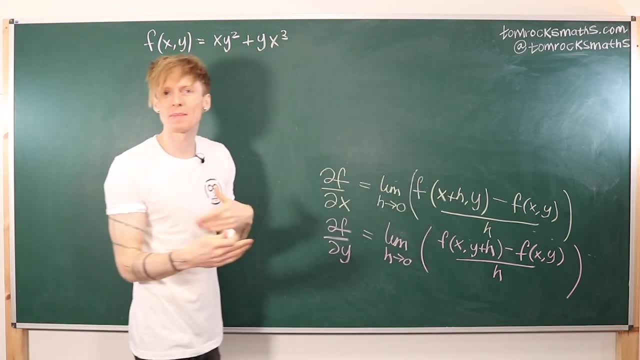 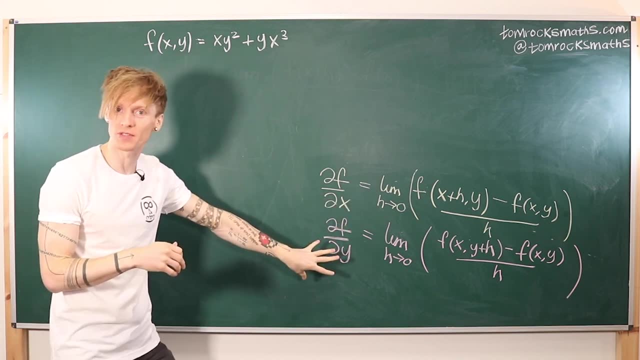 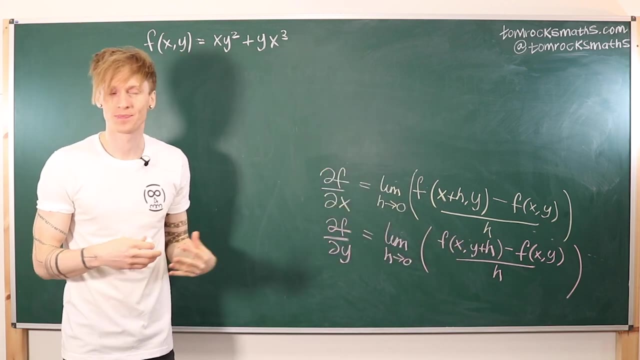 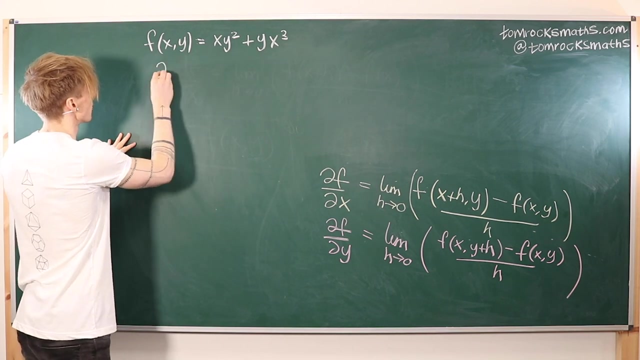 y doesn't change. So that means you can basically treat y as a constant. And similarly, when you do your y partial derivative, x isn't changing. Therefore you treat x as a constant. So if f of xy is xy squared plus yx cubed, if we calculate first df by dx, so our usual 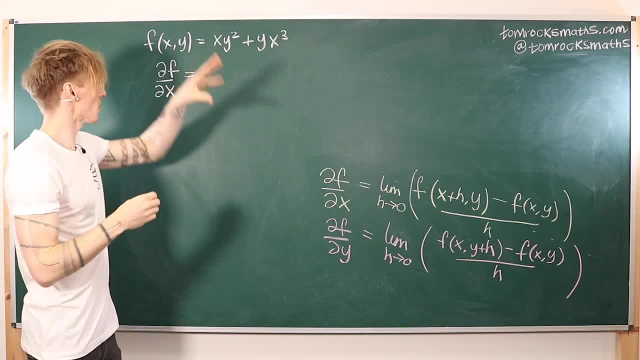 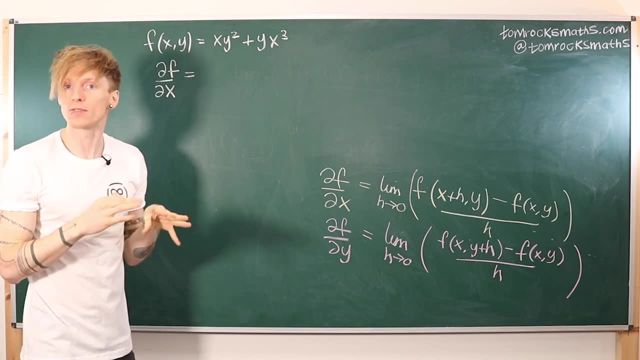 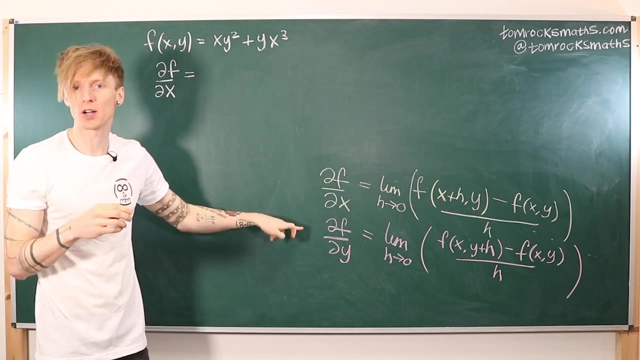 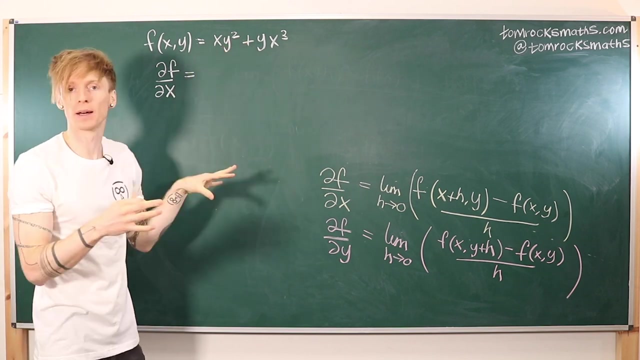 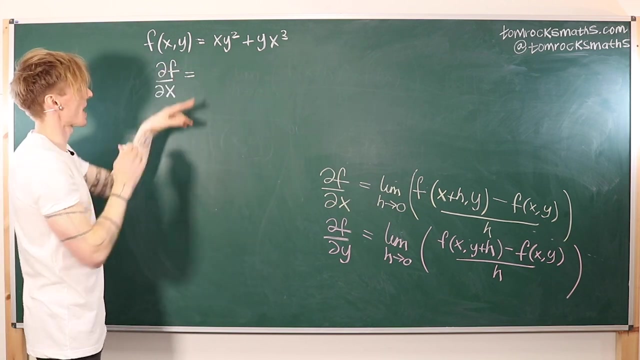 rules of differentiation apply. we still differentiate any function of x as though it is a full or standard derivative. However, remember, y is a constant, is constant in our x partial. so these y terms just treat them like any other constant. They are just a number that we just ignore pretty much. So what I mean by that is if I do df by dx. 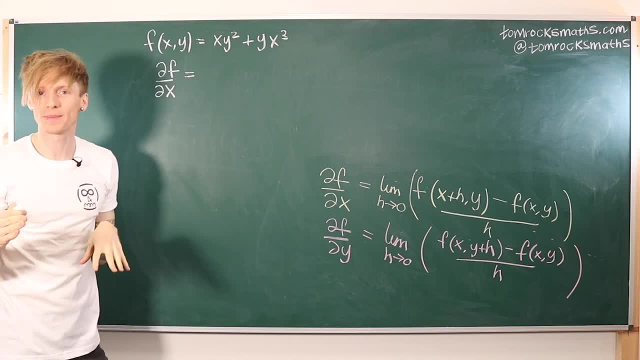 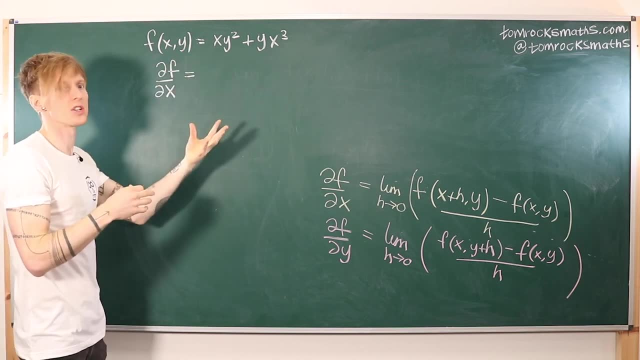 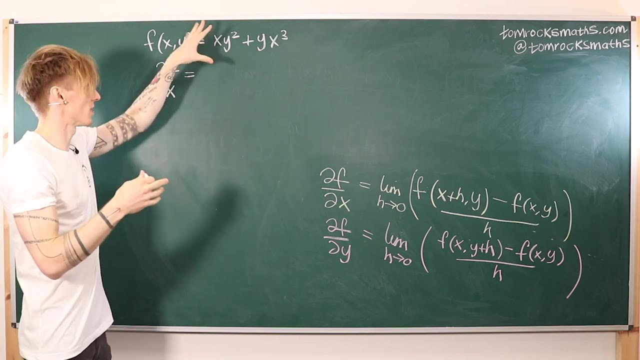 this first term, x times y squared. when y is constant, this is just constant times x. So when I differentiate a constant function times x, I just get the constant. So the derivative on x behaves as normal. the derivative of x is just 1, and then I'm still. 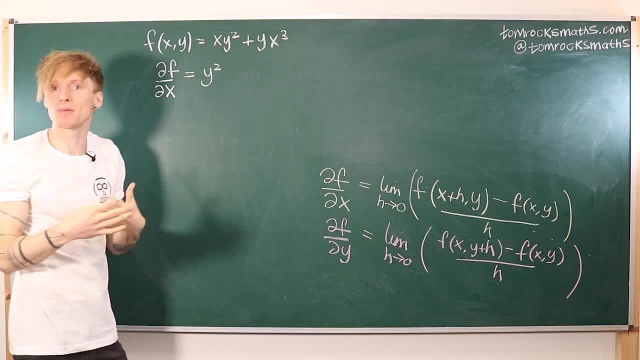 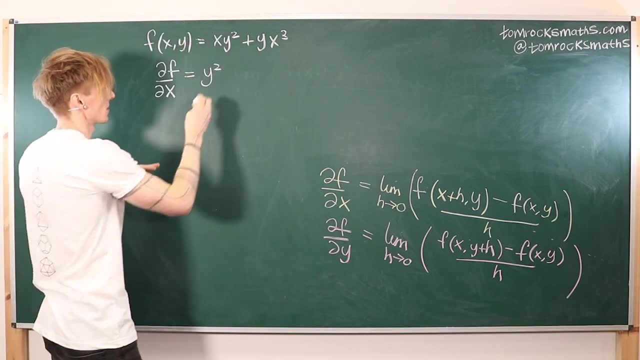 multiplying by my constant, which here just happens to be y, squared, The next term, the y, is again constant. so I just keep that. and then what's going to happen is I differentiate x by dx. So I just keep that, and then what's going to happen is I differentiate x by dx. 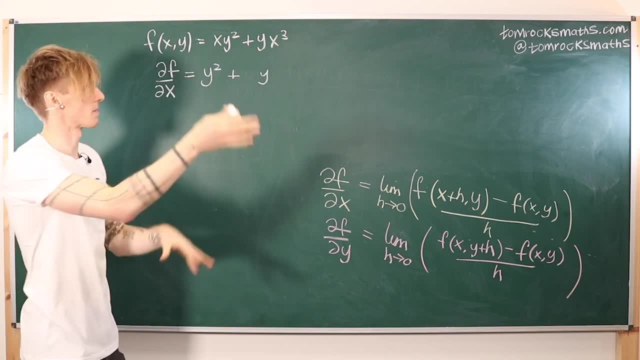 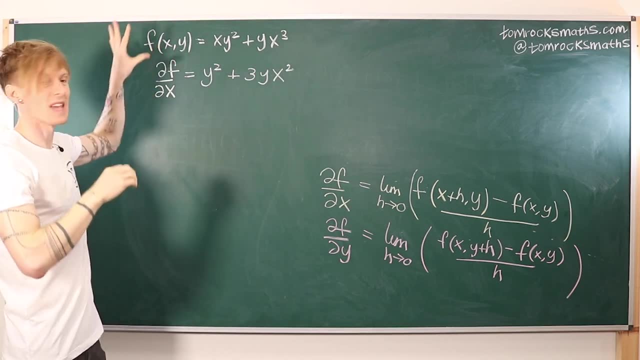 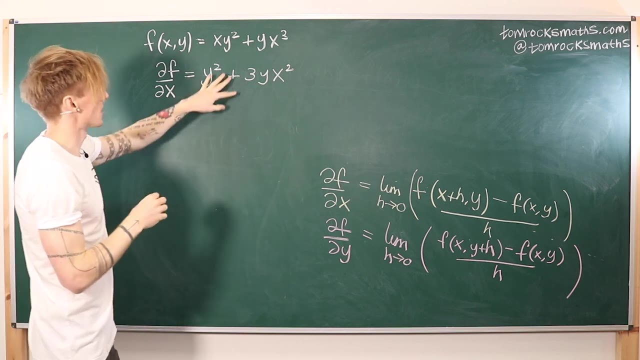 x cubed exactly as I would normally. so I bring the 3 down, bring the power down, reduce the power by 1, x squared, So the x partial derivative is just y squared, because this is linear. in x, y is constant, plus the cubed term becomes a squared. bring the 3 down and again, just leave. 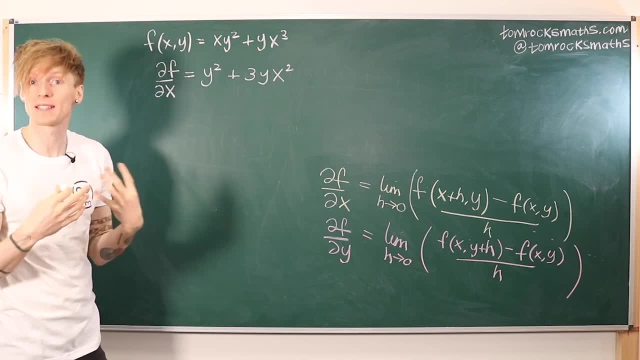 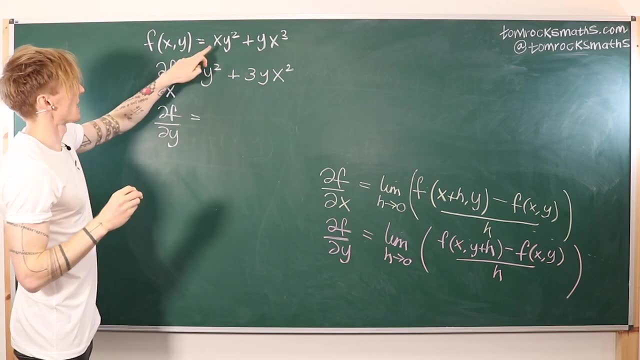 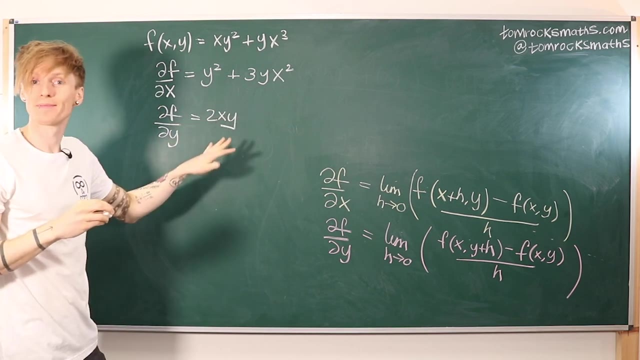 the y there because it's a constant. Now the y derivative is very similar, but this time we just treat x, x as a constant, So the x is constant. I've got a y squared, so if I differentiate y squared I get 2y. So overall the x remains where it is. I get 2xy. And then the next term. 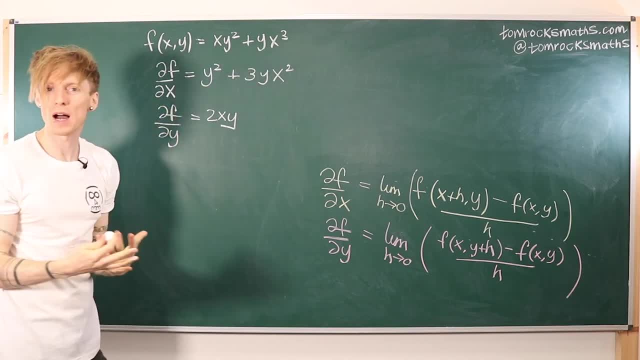 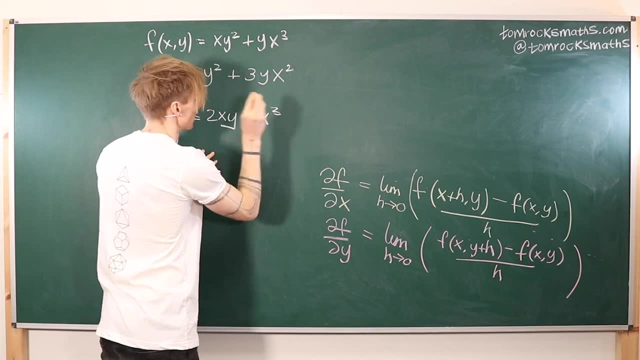 so x again is constant. this is just constant times y. so a linear function in y just gives me the constant, which here would just be x cubed, And that's pretty much it. So I've got a y squared. so if I differentiate y squared I get 2y. So overall the x remains. 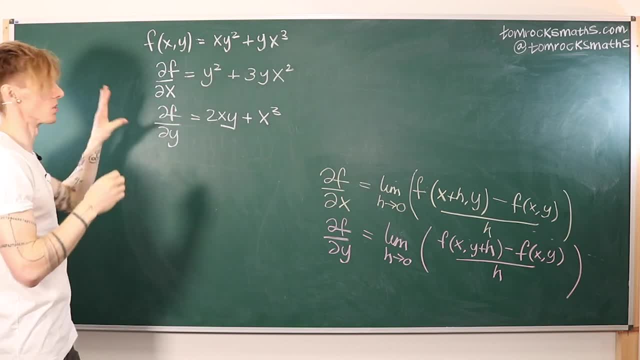 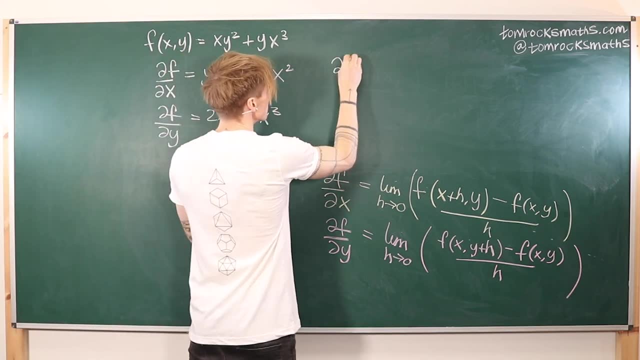 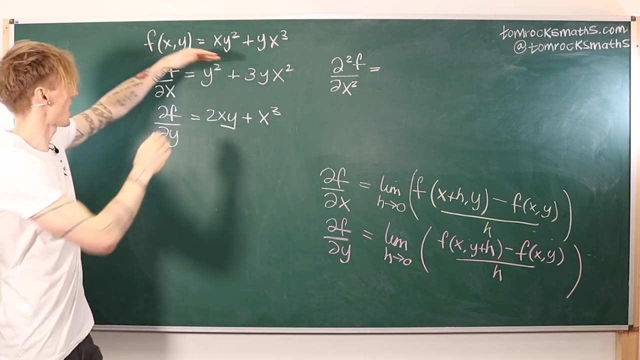 be our partial x derivative, and this is our partial y derivative. Now we can go a little bit further. we can calculate the second order derivatives, so d to f, by dx squared, And so that just means take this derivative here, df by dx. 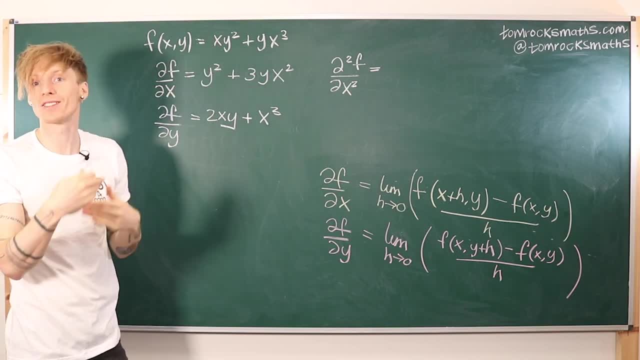 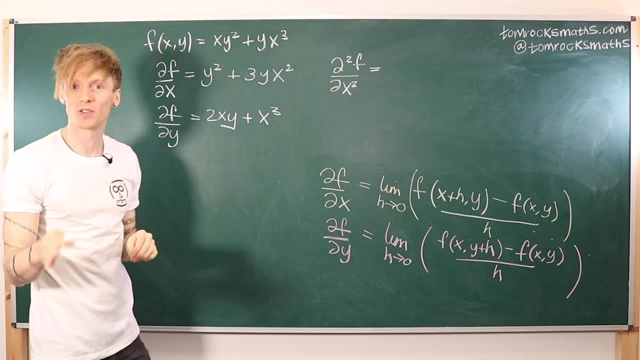 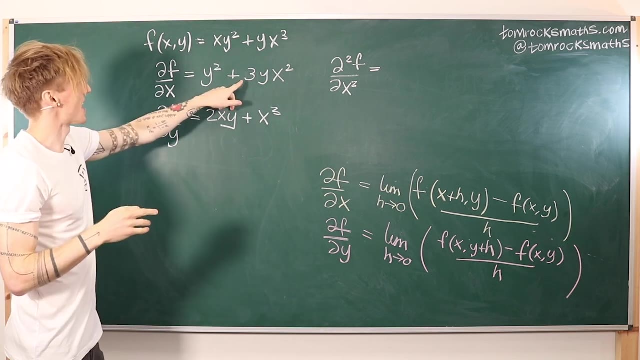 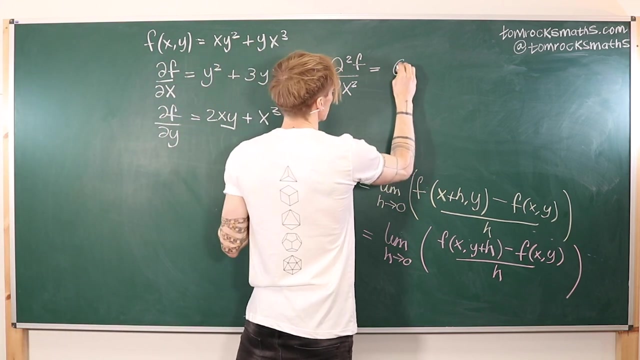 and differentiate again with respect to x, where we remember y doesn't change. so y is a constant. So this one, the first term, is a constant- differentiates to give 0.. And then if I do my x derivative on x squared, the 2 comes down, so I get 6yx. 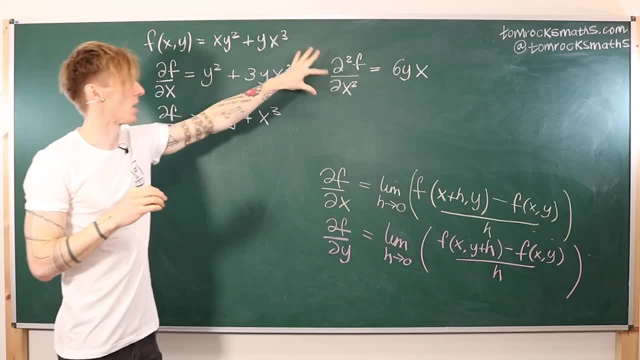 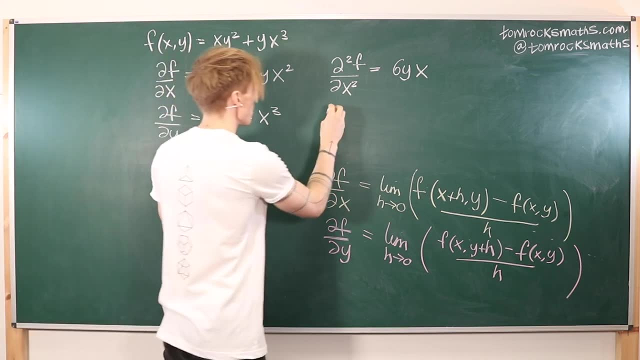 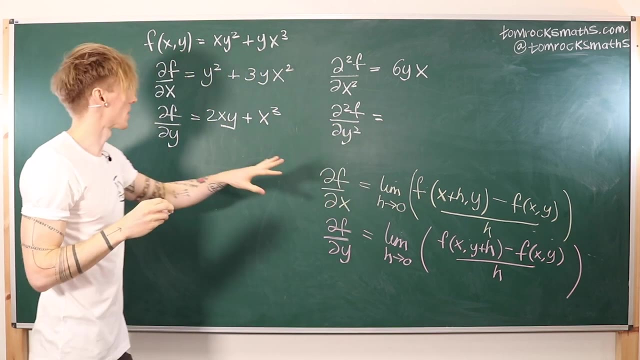 So that is my second x partial derivative of the function f. We can also calculate our second y derivative in the same way, So d2 f, dy squared, So that is going to be the y derivative of df by dy, remembering that x is a. 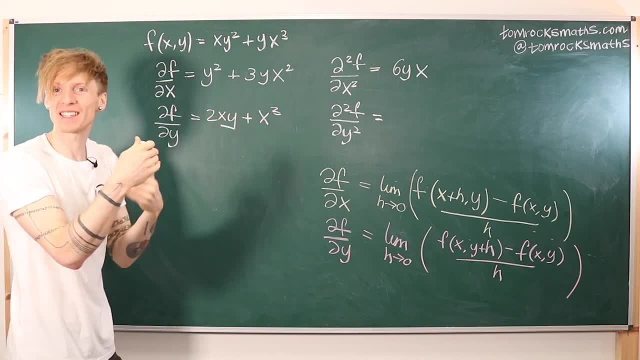 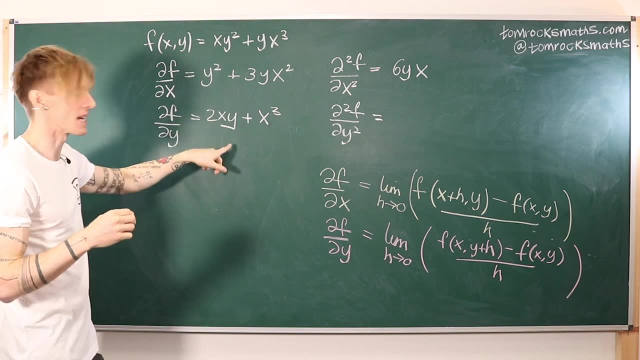 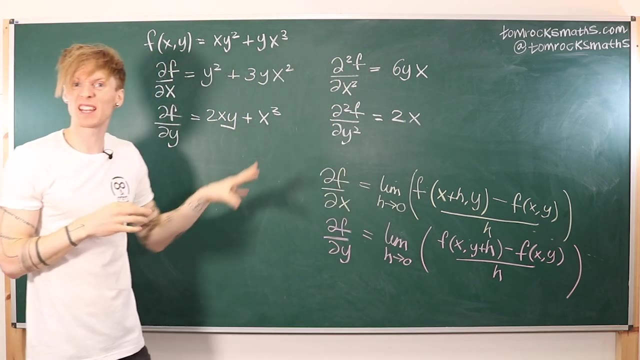 constant here. So this x cubed term goes to zero because it's just the derivative of a constant, and here again x is the constant. We differentiate the linear function of y, so we're just going to get that 2x. and we could carry on. we can calculate higher and higher derivatives, we can even mix the. 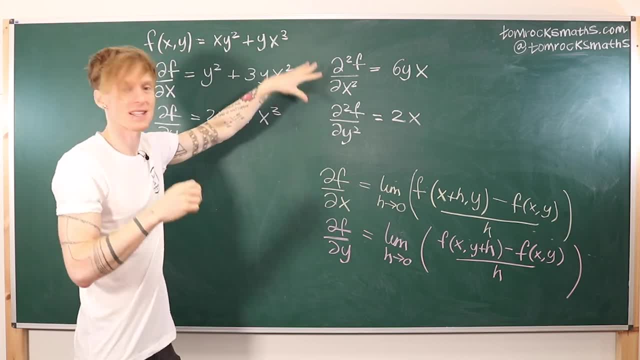 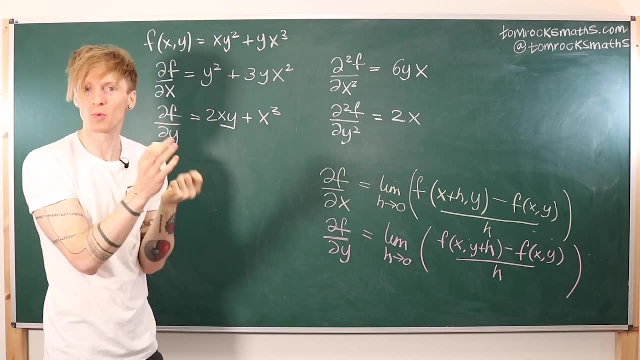 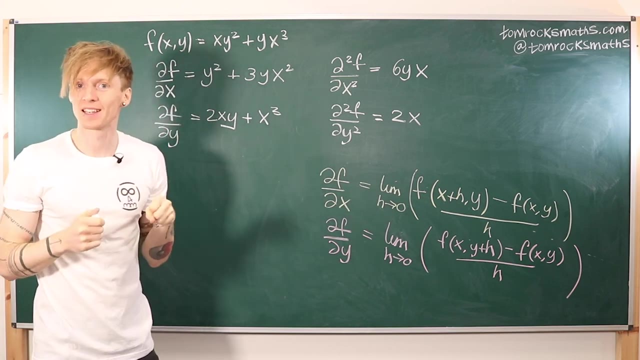 derivatives. so we could do d2f by dx, dy, or even d2f by dy, dx, where you're changing the order. so one of them means do x derivative first, then the y derivative, and the other one would mean y derivative first, then x derivative, and I do recommend trying this out for yourself. 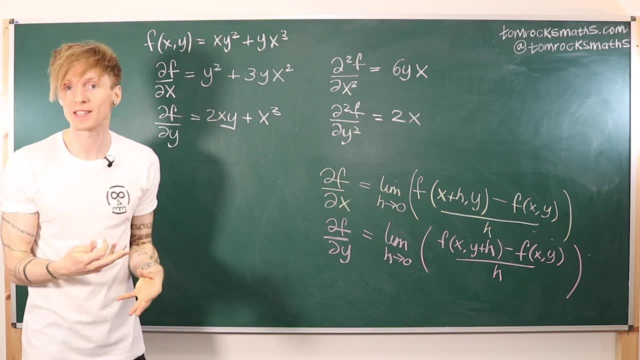 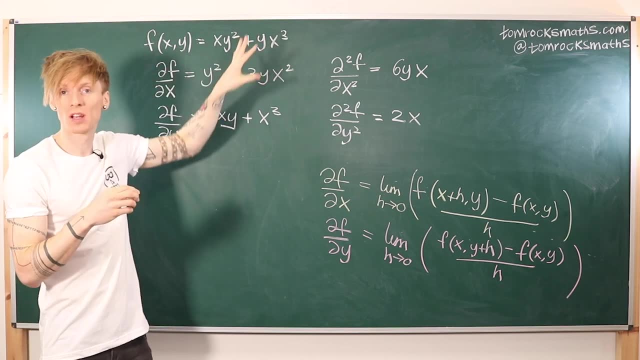 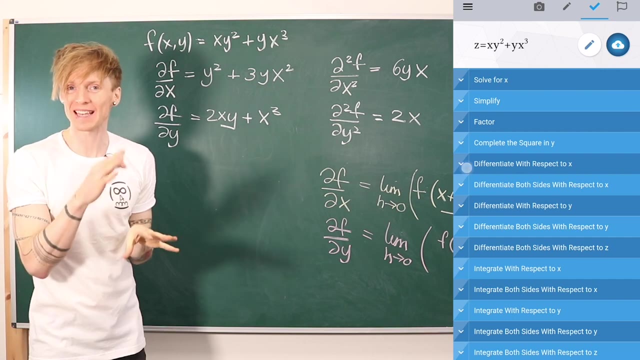 to get practice with doing partial derivatives of higher orders, maybe with mixed derivatives. so just pick any function f of x, y. you can plug it into the maple calculator app and it will automatically tell you the x and y partial derivatives of the function once you enter it. 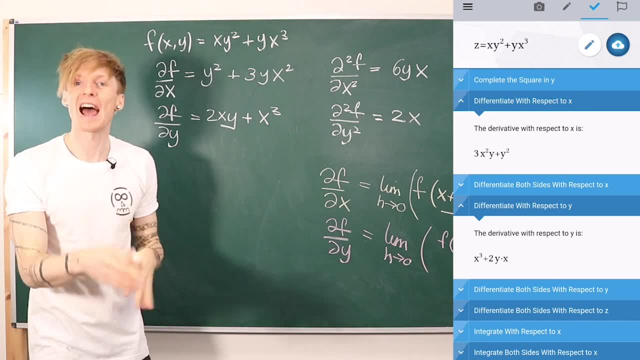 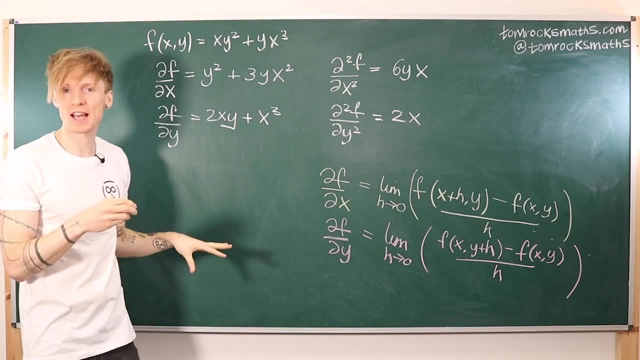 into the app. so you should do it yourself first, and then you can use the app to check your answer, you and sort of mark your own work and see if you're beginning to grasp how partial differentiation works, all of the other rules about differentiation that you may. 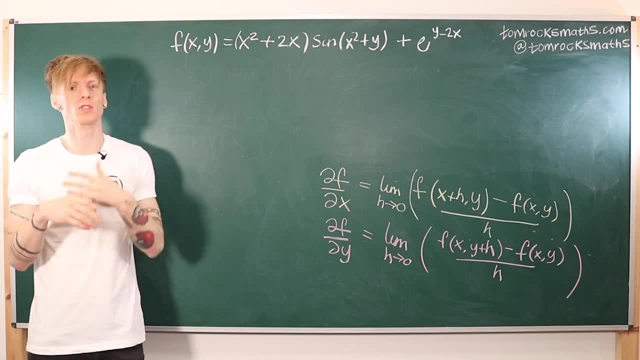 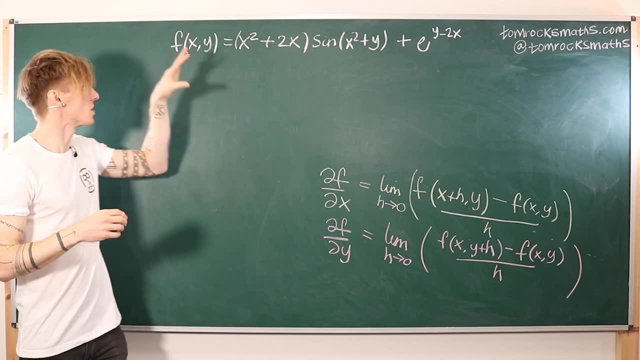 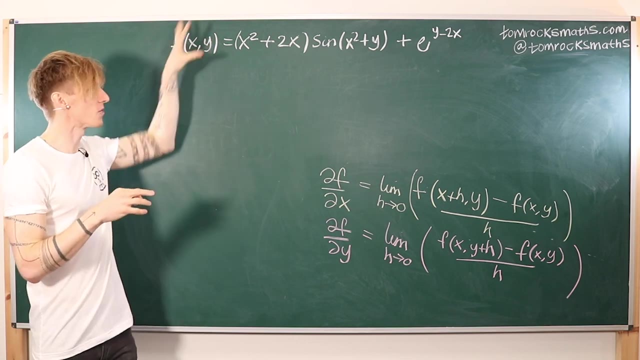 have learned, for example, the product rule, the quotient rule, the chain rule. these all still apply when doing partial derivatives. so I've got another example here which is a little bit more complicated, but we'll go through the first partial derivatives to give you a feel for how the product. 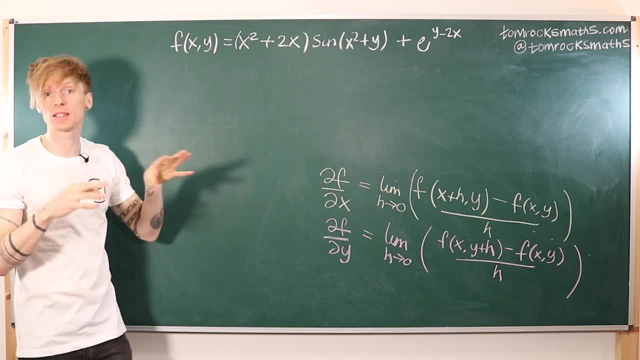 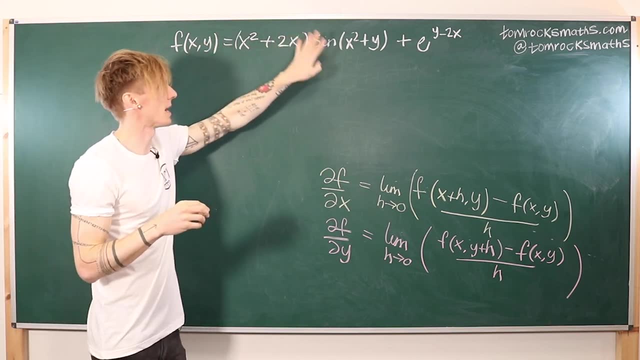 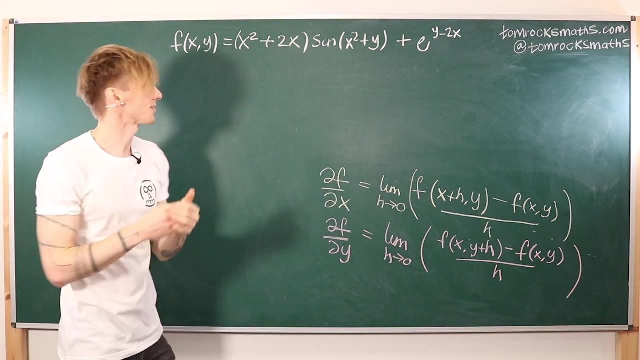 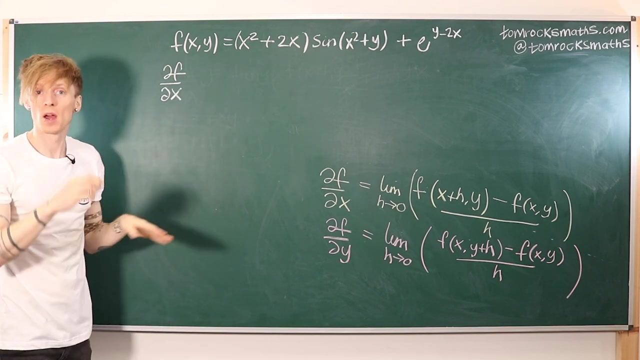 quotient and chain rules work in this context. so f of x, y is going to be x squared plus 2x, all multiplied by sine of x squared plus y plus e to the y minus 2x. so first of all let's calculate our x partial derivative, df by dx. we remember that y doesn't change. y is now a partial derivative. so 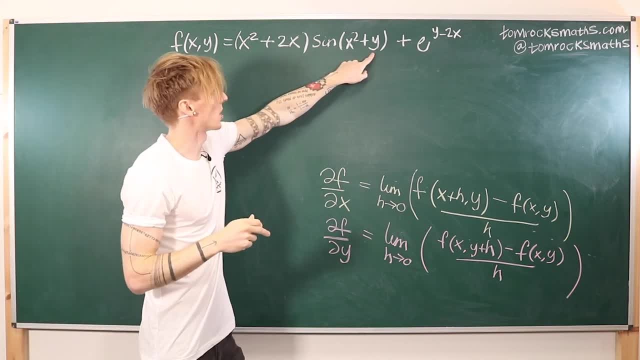 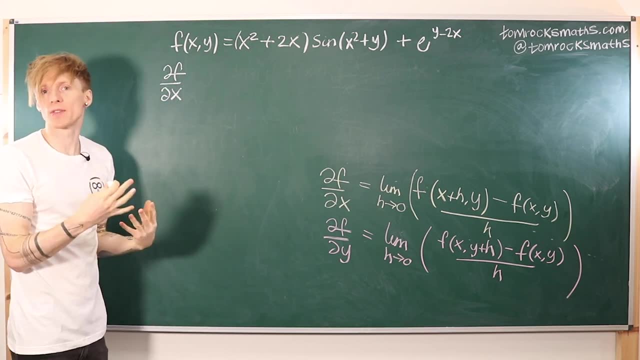 if we look at the Hehe now, we get 1 over 2 because we have 2x squared plus 2x squared plus 2x squared. so if we try that again in the previous example, what we see is that y is now a constant. so this is: 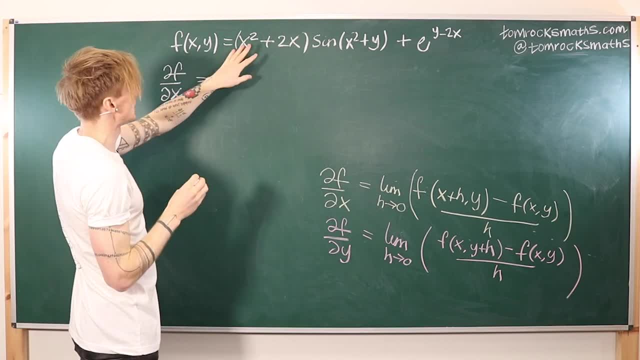 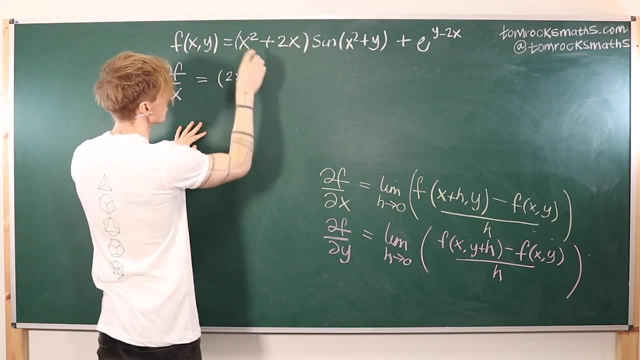 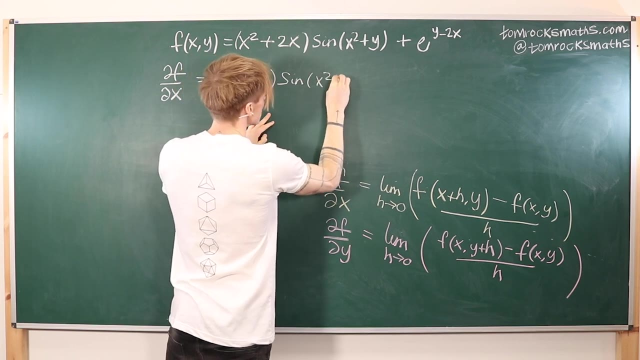 just now a constant, as is the y in the exponential. now I still need to do the x derivative using product rule and also a chain rule as well. so the first term, let's do a product rule. so let's the second term, which is unchanged. Now I want to differentiate the second term. 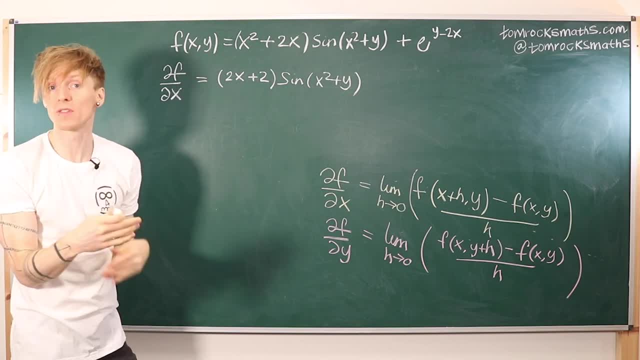 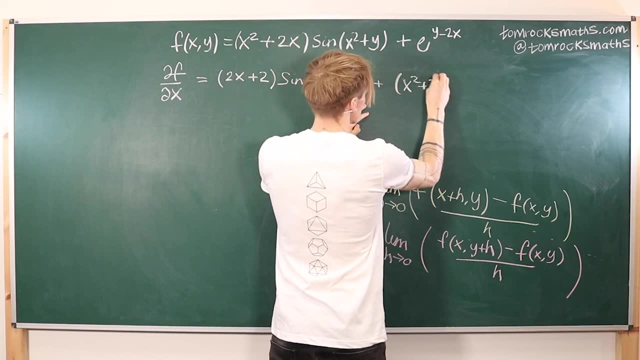 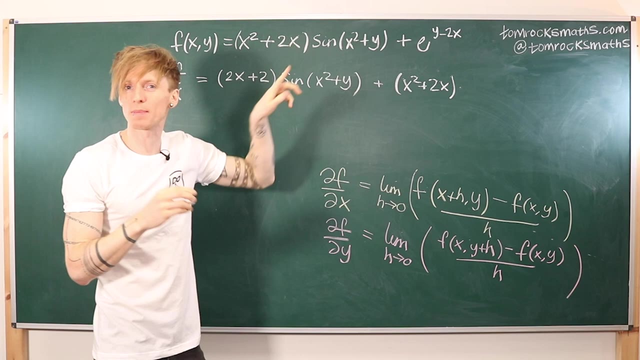 and leave the first term unchanged, as I would for any normal product. So that will give me plus x squared plus 2x multiplied by the x derivative of sine of x squared plus y. So I'm going to have to do a chain rule as well. so we 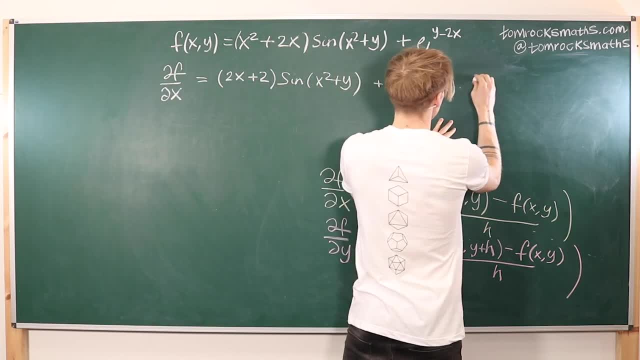 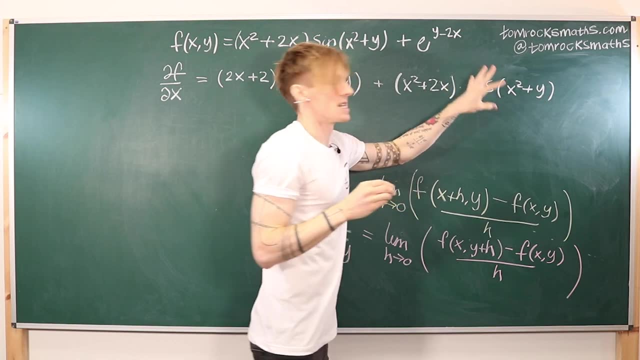 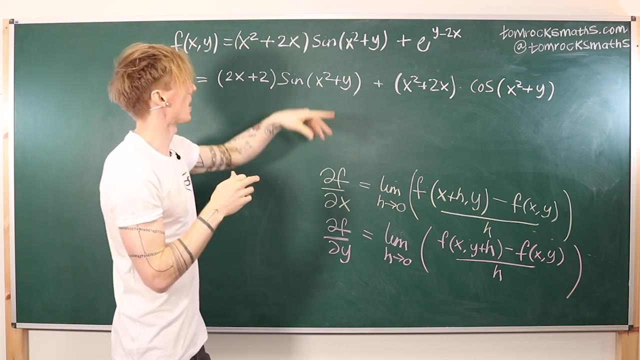 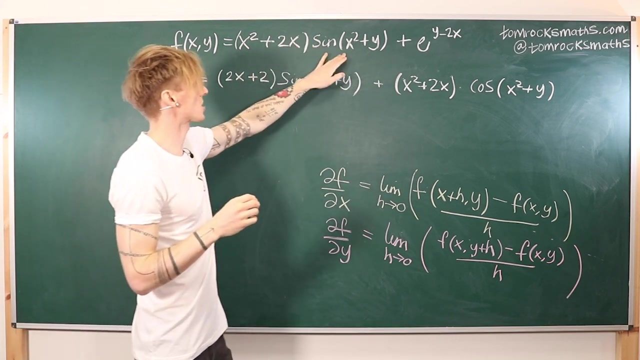 differentiate sine, which gives us cos of x squared plus y. Now, having differentiated the sine, we get cos. but then the chain rule says I have to multiply by the x derivative of the argument of sine. So I've got x squared plus y. y is a constant in this situation, because I'm doing an. 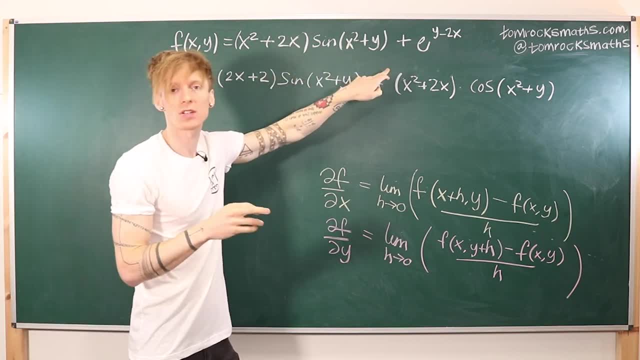 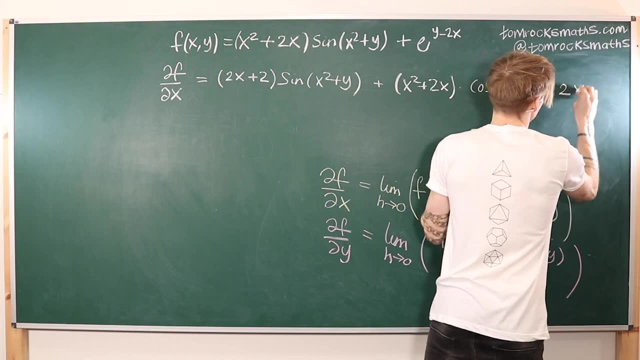 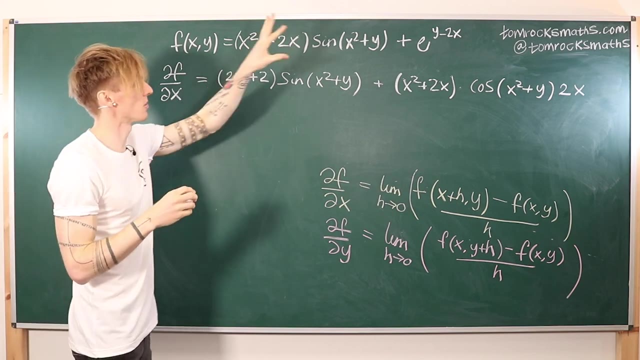 x-partial, so x squared plus constant. if I differentiate that with respect to x, I just get 2x, and that will be the product rule done on that first term. Now we also have to differentiate the exponential. so what I'm going to get here is the exponential squared plus sine and then the 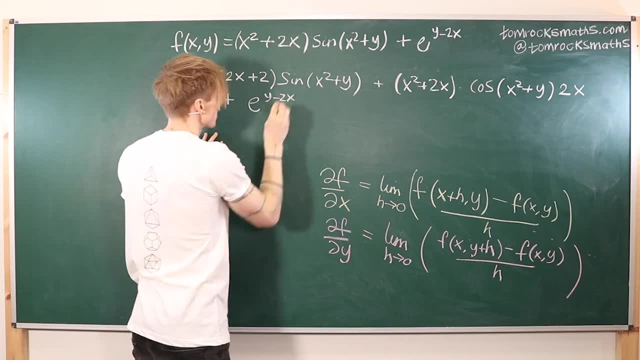 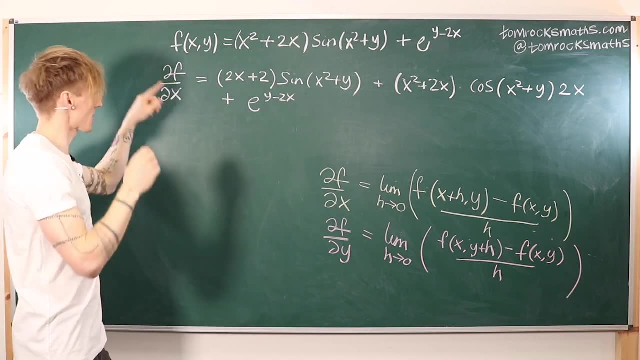 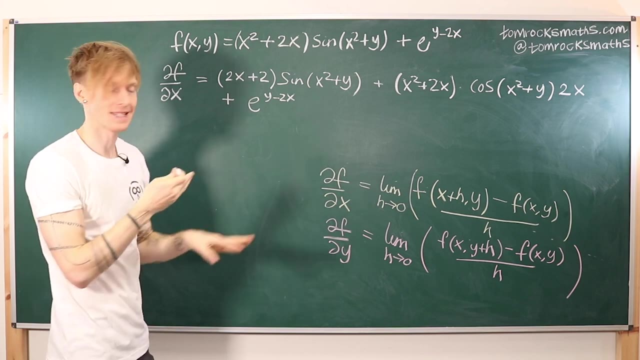 unchanged. so e to the y minus 2x and then from the chain rule. I have to differentiate the argument, so I need to do the x partial derivative of y minus 2x. y is a constant, so that disappears and we just get minus 2 from the chain. 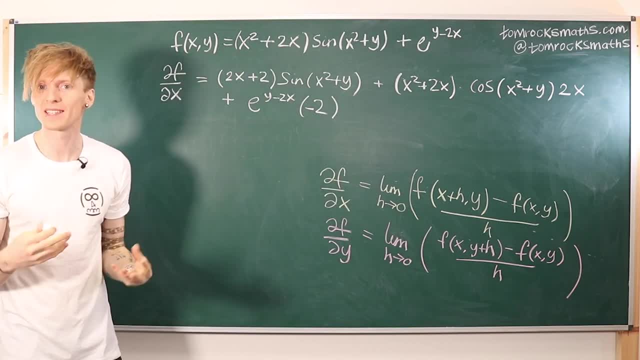 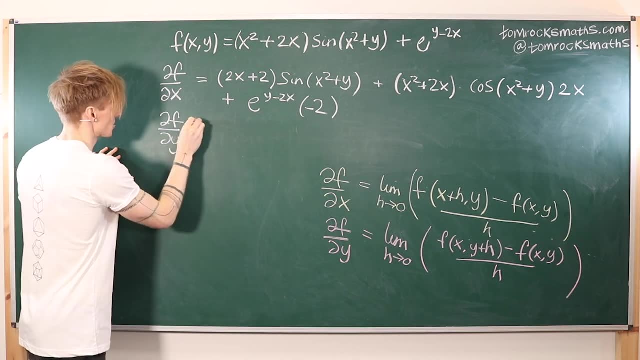 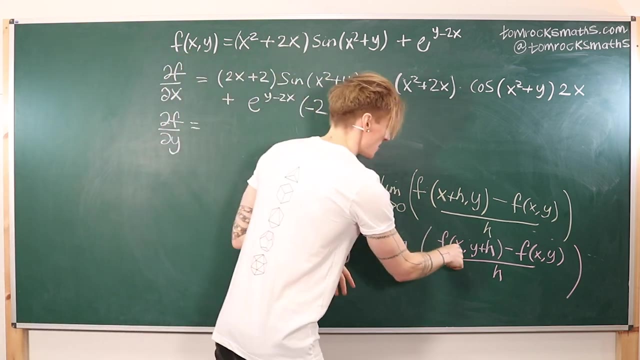 rule. Finally, if we now do the partial y derivative in much the same way, this one is actually a lot easier, because we remember that when we're doing a y partial derivative, we've got over here that x isn't changing, x is constant. So 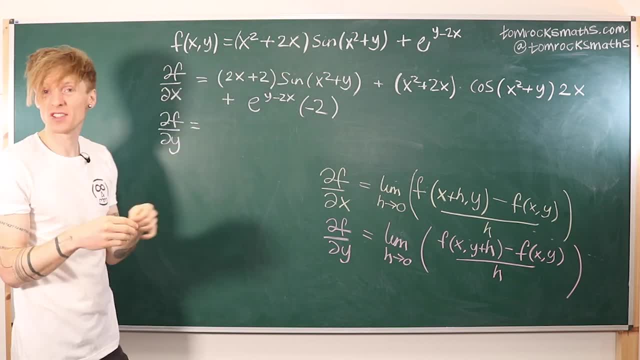 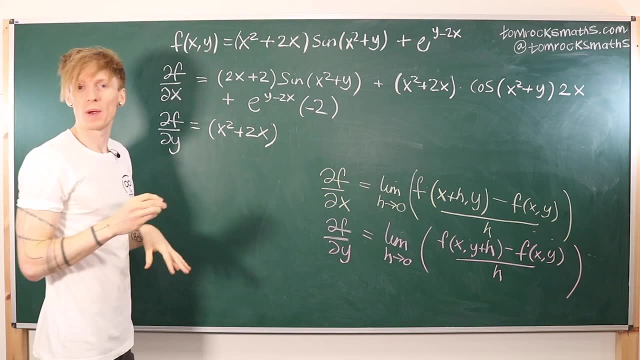 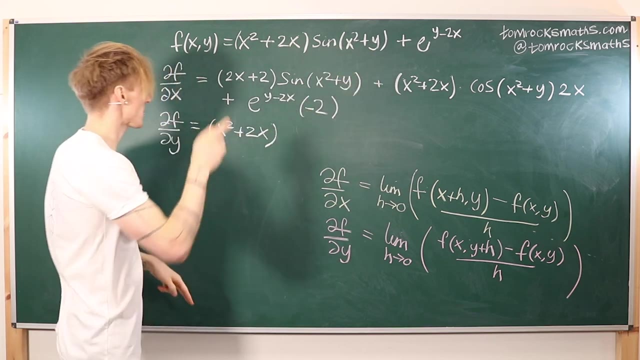 this whole term. x squared plus 2x is just a big old constant, so that just stays where it is. and now what we actually differentiate is the sine term here, because that has a y dependency. So the derivative of sine gives me cos of its. 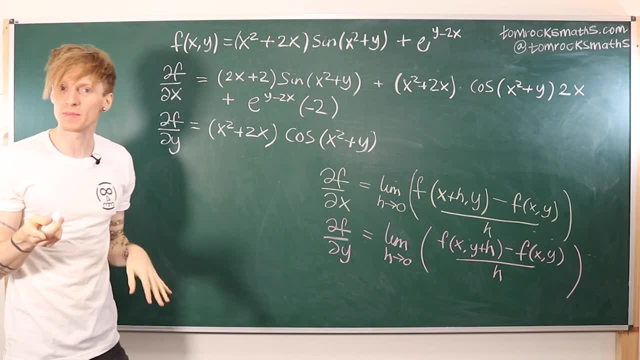 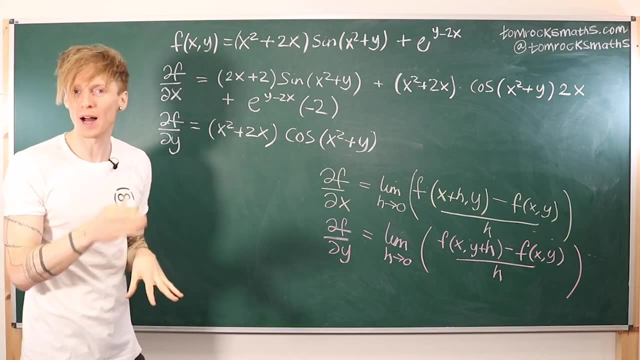 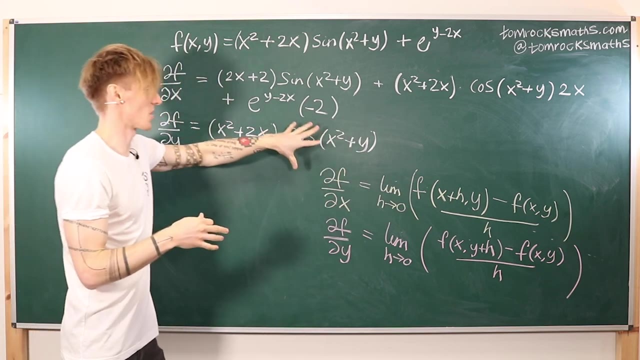 argument, and then the chain rule tells me to differentiate the argument. but when we're doing this with respect to y, x is a constant, so the y partial of x squared plus y is just 1.. So you don't actually get an additional factor and